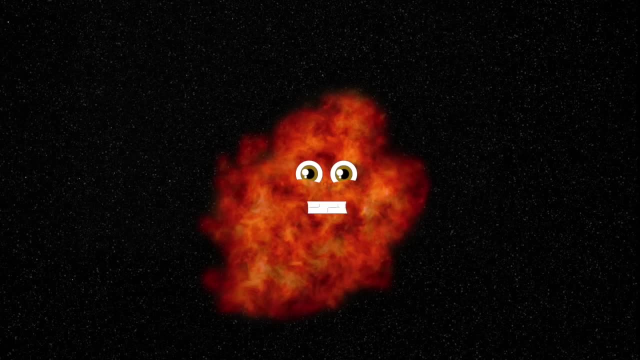 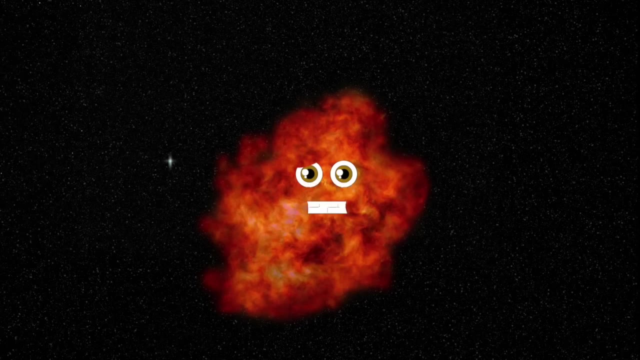 high density and a very low temperature. This combination creates a gas, molecular hydrogen. That's primarily what I'm made of, along with cosmic dust within. When the force of gravity exceeds the outward push of gas, the pressure is so great that I can't help it and start to collapse. 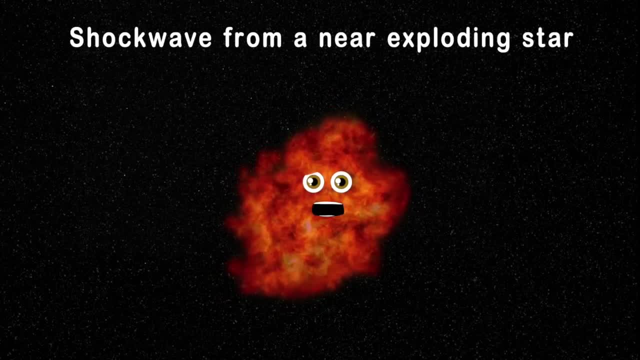 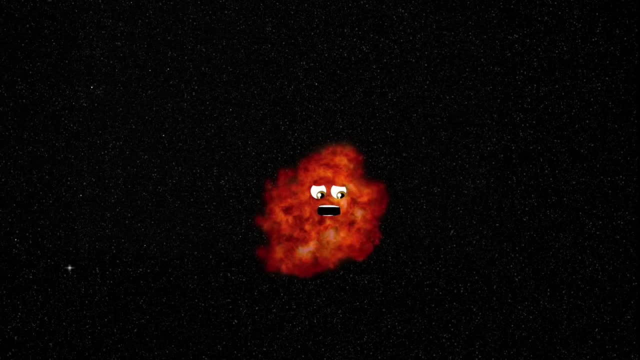 which is caused from a shockwave from a near-exploding star. Oh, when two molecular clouds collide now, isn't that bizarre? When the gravity's too strong, I break apart into smaller clouds. Each cloud is a star's beginning in which I am very proud. 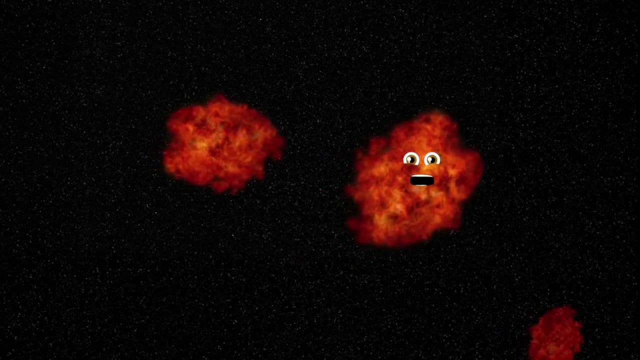 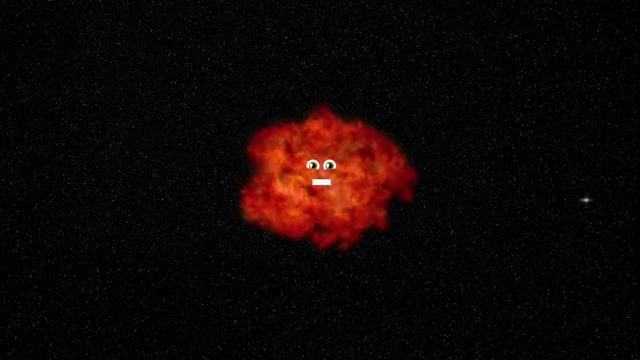 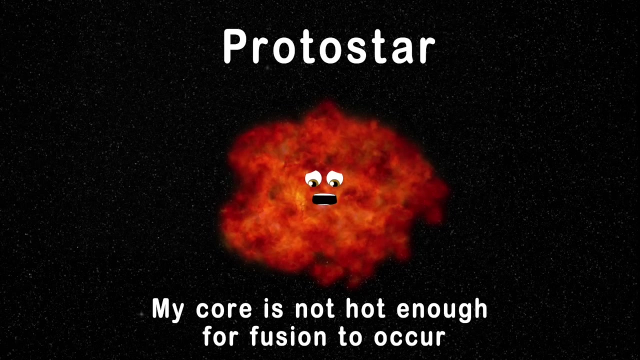 Proto-stars are the name of the clouds that do break free. Let me introduce a proto-star. that was a part of me. Hello, there, I'm the beginning of any kind of star. Let me introduce myself to you. I am a proto-star. My core is not hot enough for fusion to occur To achieve that. 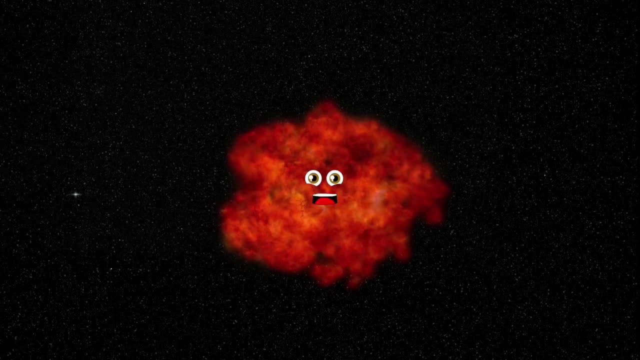 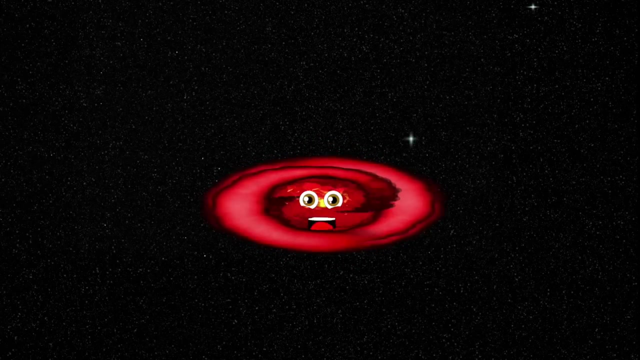 level of stardom. that process is a chore, Everything I do. when I break free from my molecular cloud, I start to spin until I form this disk around me. you see now, As the disk rotates, I produce a strong magnetic field. 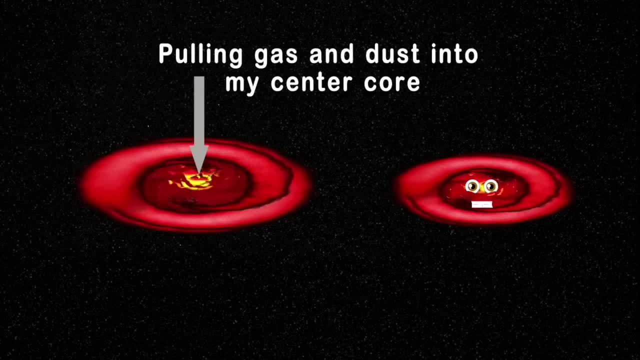 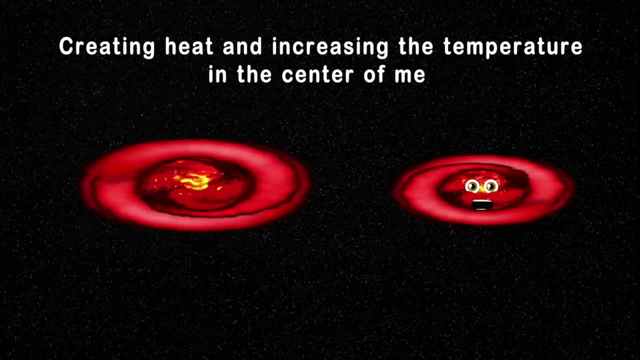 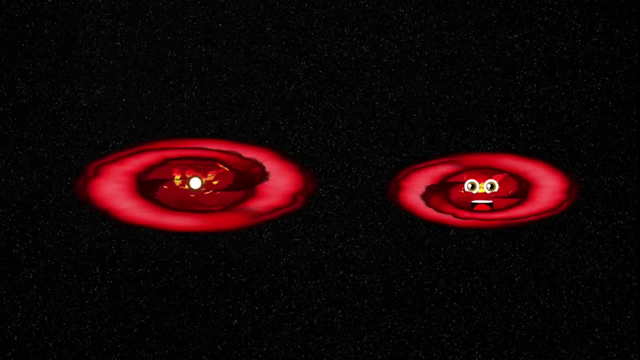 pulling gas and dust into my center core. as I reveal, The infalling gas releases a kinetic energy, creating heat, increasing the temperature in the center of me. At this point, I can transform into a hydrogen burning star, which is when the nuclear fusion starts. It's 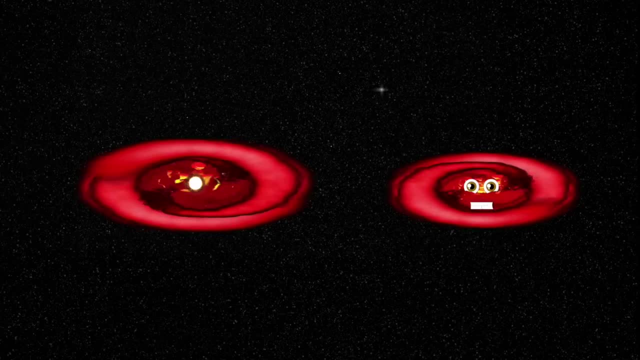 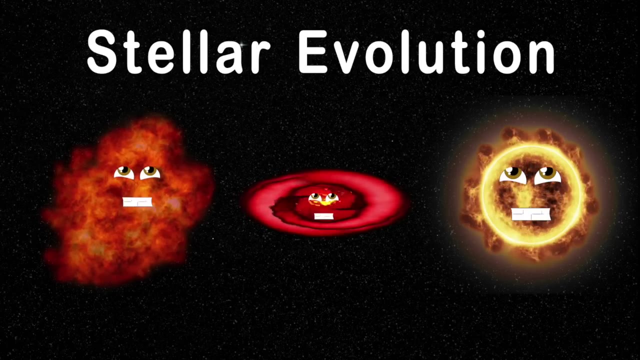 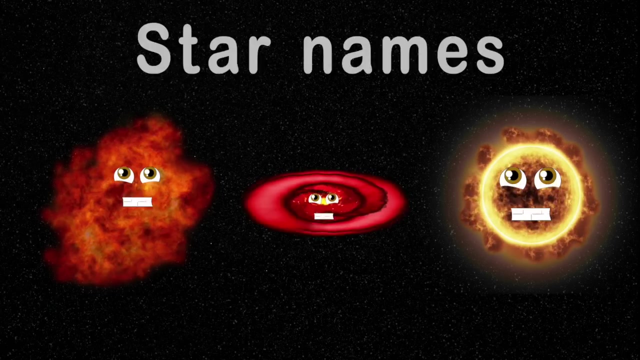 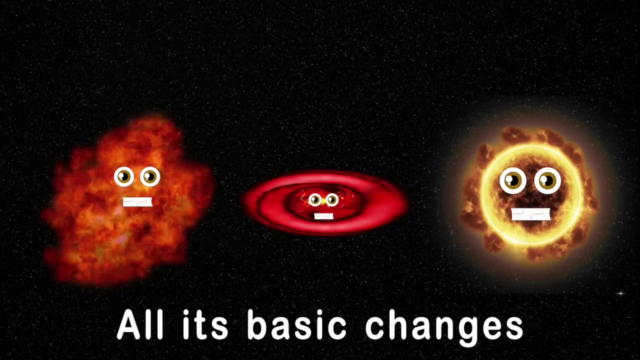 the 1,2,3,4,5,6,7,8,9,9,10,10,11,12,13,14,15,16,17,18,18,19,19,20,22,23,25,26,27,28,29,30,31,32,34,34,35,36,37,39,40,40,38,39,41,42,35,37,42,34,36,40,39,42,44,35,36,40,40,45,44,45,47,47,49,49,50,50,50,50,50,51,51,52,52,52,53,53,53,53,54,56,56,57,67,58,58,59,61,52,53,55,57,68,59,59,60,61,62,63,64,63,63,64,64,65,67,69,79,80,.